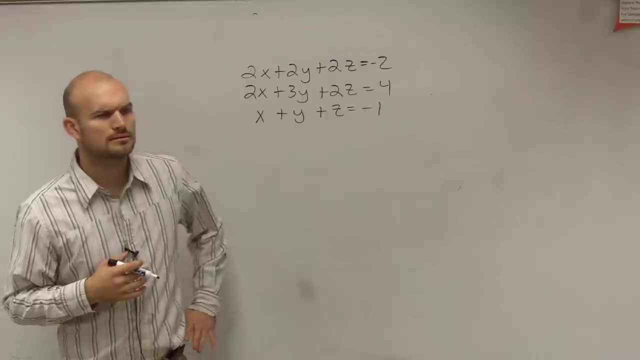 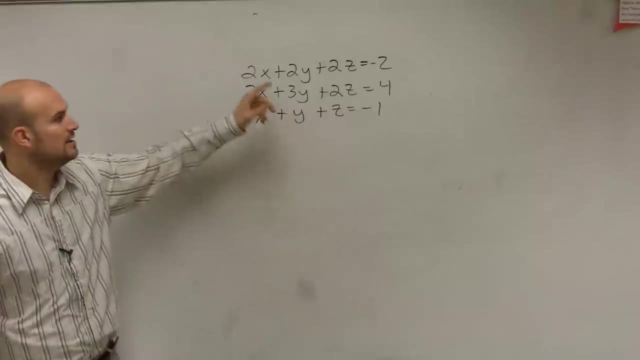 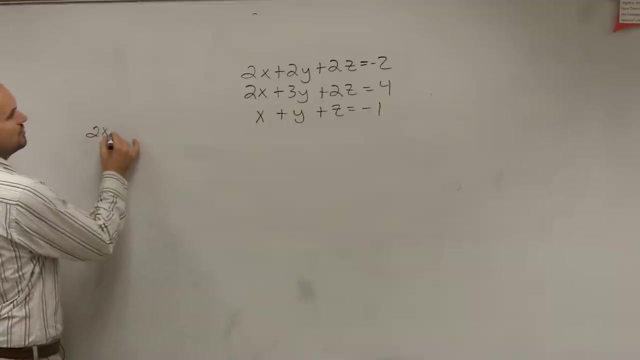 So let's go and eliminate our Y. If I want to eliminate the Y between the first and the third, let's write out the first and the third equation. So I'm going to do 2X plus 2Y plus 2Z. 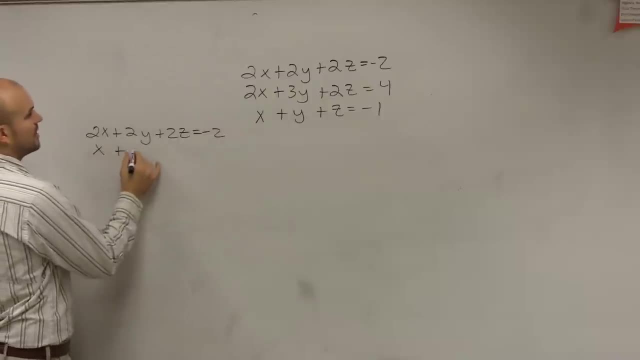 equals negative 2.. And then over here I have X plus Y plus Z equals negative 1.. So to eliminate the Y, what do I need to do? I need to multiply my second equation by negative 2, right, If I wanted to add them, I could multiply it by 2 and then subtract them, Or I could also divide the top. 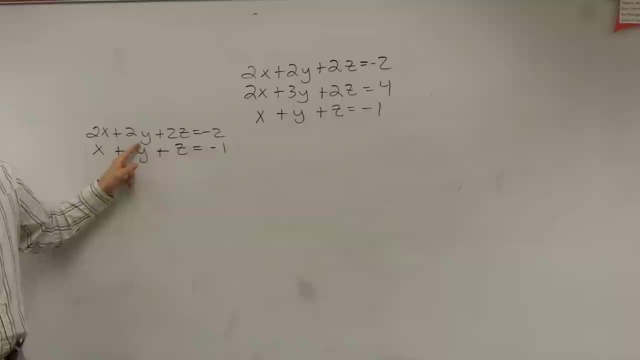 equation by. I could also divide it by negative 1, right, Or divide it by or, I'm sorry, divide it by negative 2.. So, but let's just multiply this by negative 2.. So I'm going to do 2X plus 2Y plus Z. 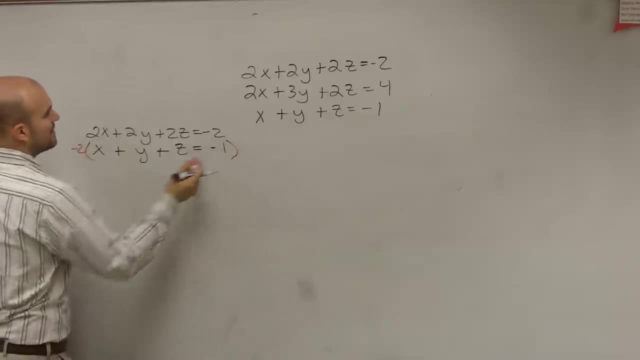 equals negative 2.. Just make things simple. So I'm going to multiply everything times negative 2.. So therefore I get. so let's label our equations 1, 2, 3.. So right now I'm doing equation 1 and 3.. 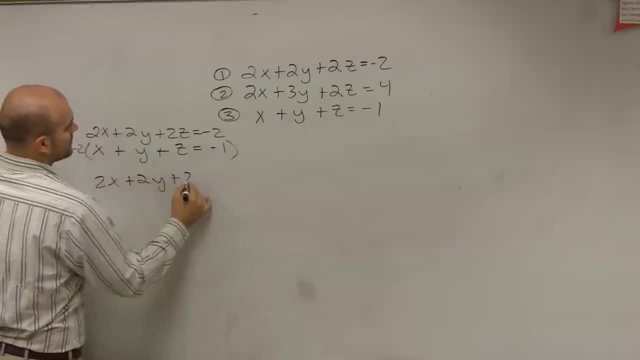 So I do: 2X plus 2Y plus 2Z equals negative 2. Therefore I get negative. 2X minus 2Y minus 2Z equals positive 2. Right, Correct. Then when I go ahead and solve for this, I get 0 equals 0.. 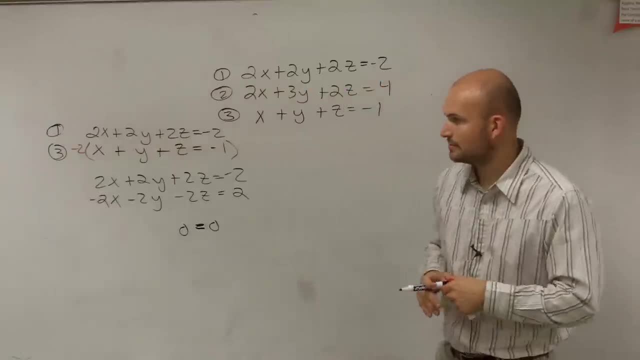 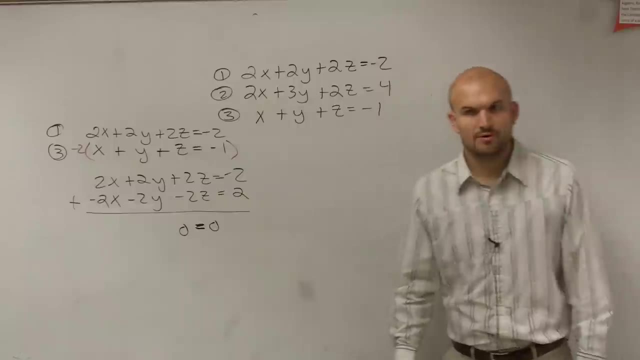 Okay, Right, When you add these up together, Because now the next step. you're supposed to add these up Now. we're supposed to get equations from this, But we get 0 equals 0. Now, ladies and gentlemen, remember what we're talking about when we're looking at. 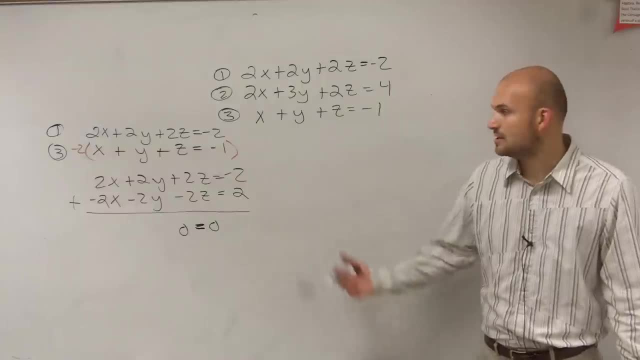 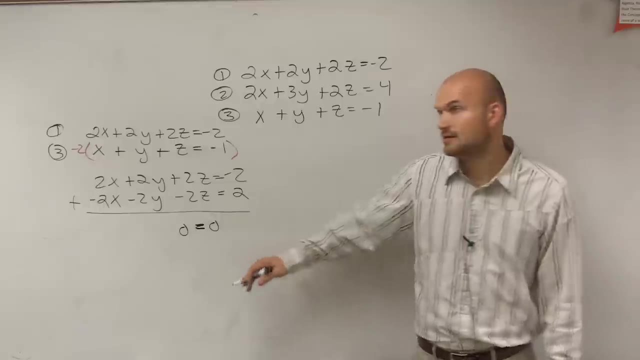 our systems with three equations. When we have something like this, what does that tell us about our solution? That we're going to have infinite many solutions, right? So let's just go ahead and take a look at equation number 2 and number 3.. 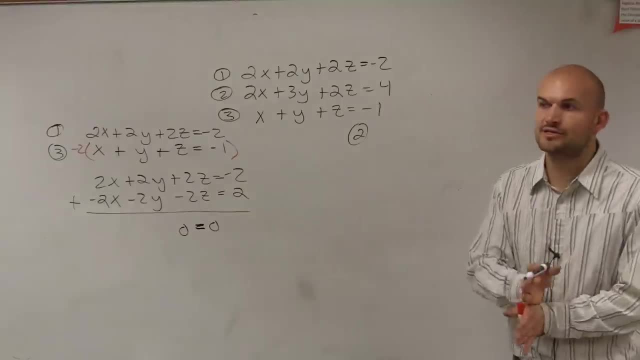 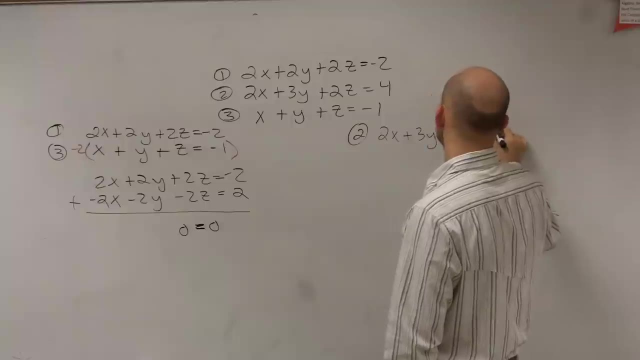 Just to make sure that we're not dealing with two lines that are exactly the same intersecting another line. So we have 2 equals 3, so we do 2X plus 3Y plus 2Z equals 4.. And they have X plus Y plus Z equals 6.. 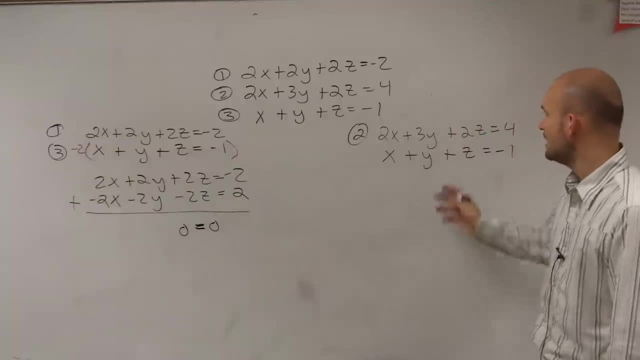 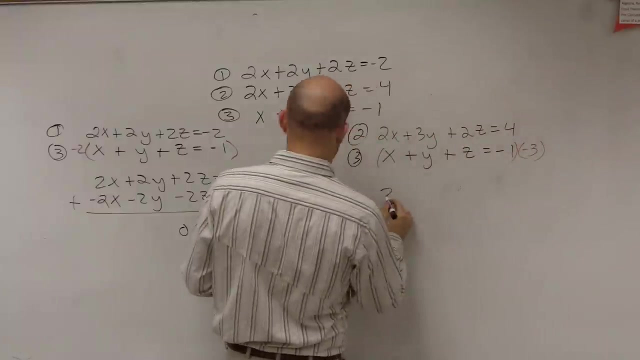 plus z equals negative 1.. And let's say we want to eliminate y. So to eliminate y on this one, we're going to have to multiply the top equation by negative 3, right? So therefore you get 2x plus 3y plus 2z equals 4.. 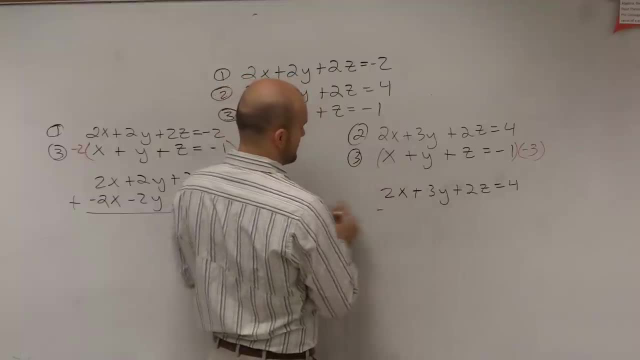 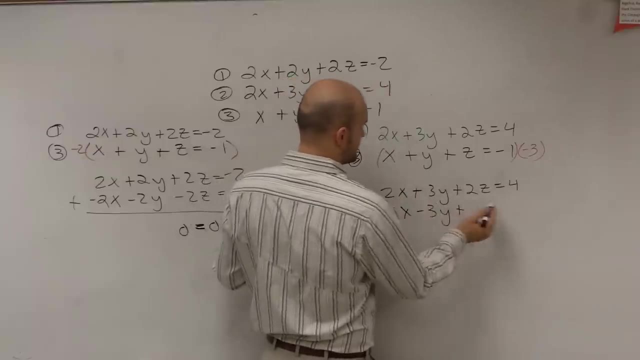 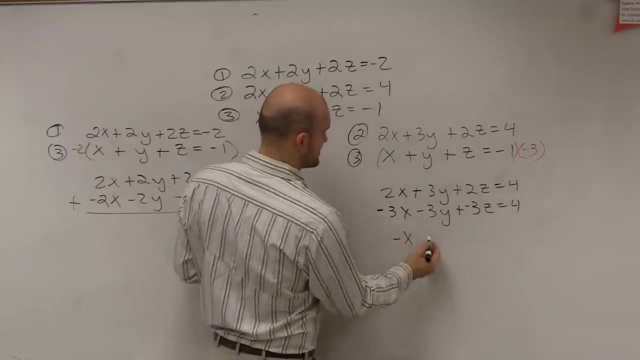 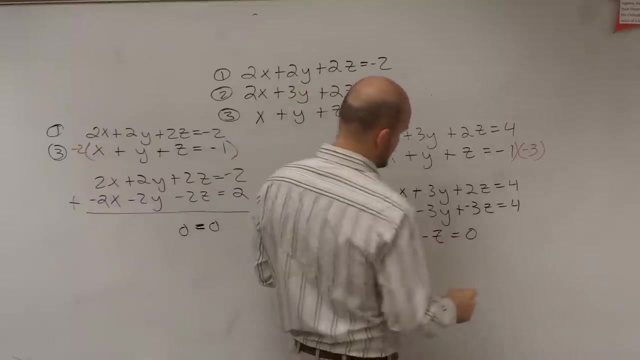 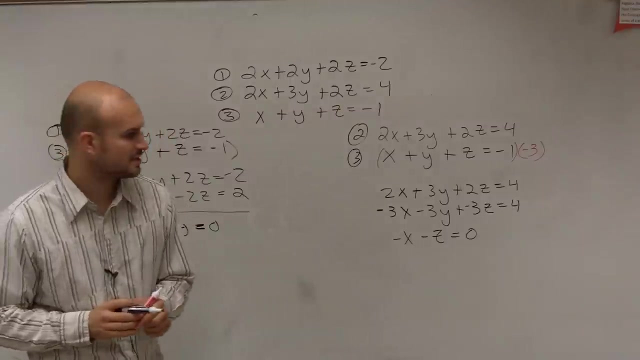 And here we get negative 3x minus 3y times a negative 3z equals 4.. So you get negative x 0y minus z equals 0. I'm just showing you guys another step. That's a positive 3, right. 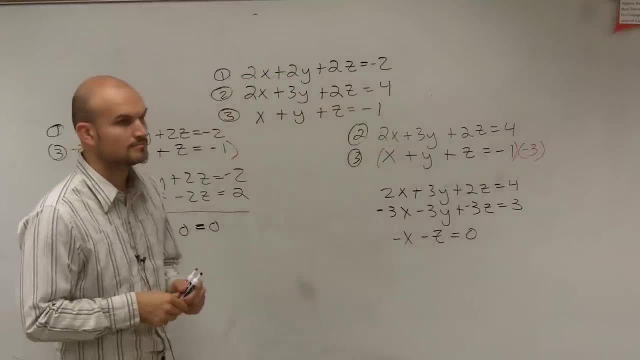 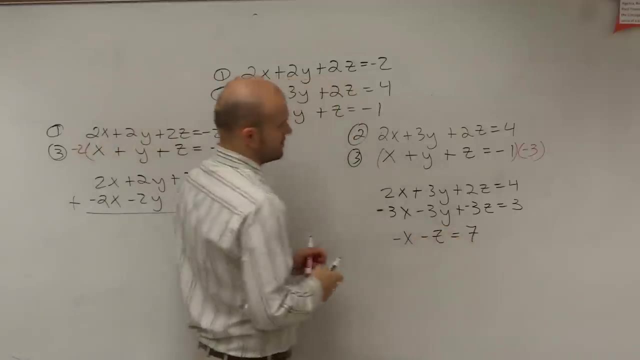 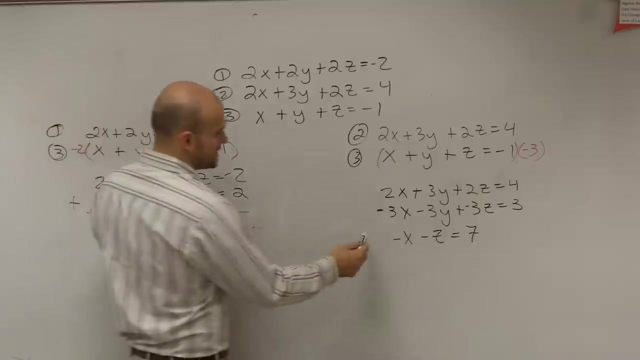 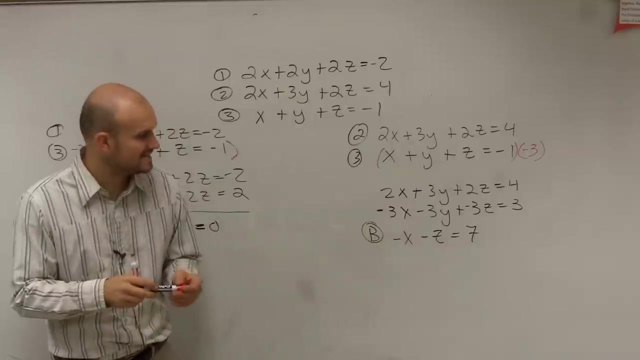 Thank you. So now, when we do a plus a, we get here we have infinite many solutions. and here we have, Let's see, Let's see Equation B: negative: x minus z equals 7.. Now let's think about this. 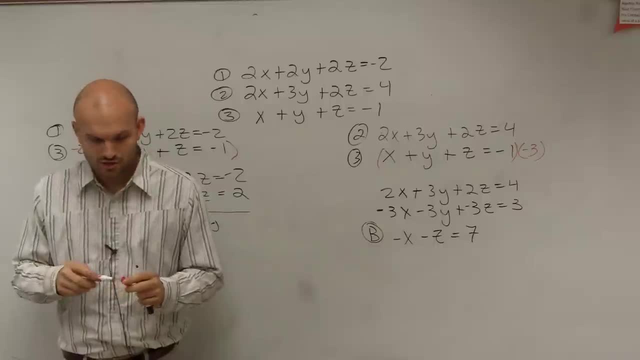 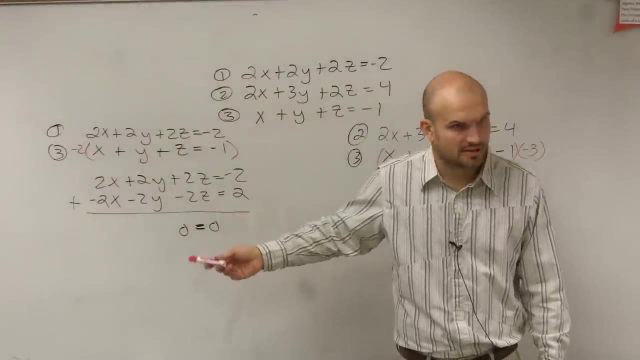 in terms of what possibilities could we do? all right, So we eliminated these two down to 0 equals 0. That always told us that we have infinite many solutions. right, Because there's infinite many things. Now let's look at this. 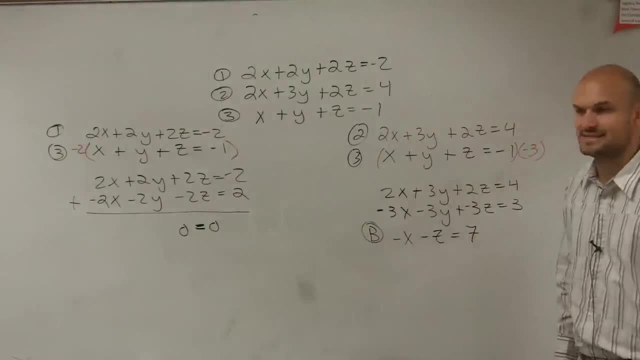 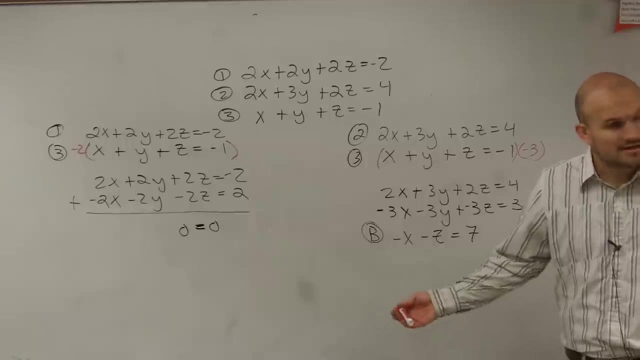 How many possibilities are there for me to take negative x minus z and get 7?? How many possible combinations are there? Infinite, Infinite, right. So this is another way. if you get to this point, you guys can see. that's why we get infinite many solutions okay. 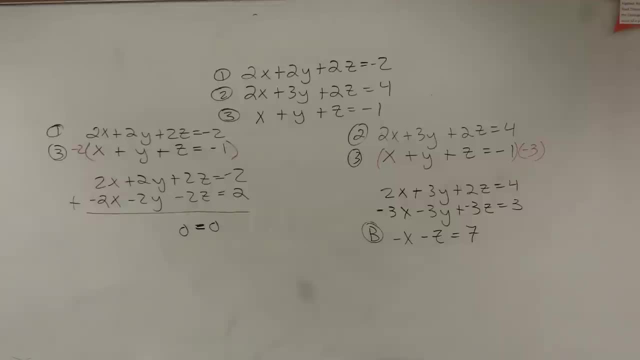 Because when you guys look up there, what you obtain is infinite many solutions. all right, Yeah, you can see, Because think about it. What are the possibility? It's like me saying what's x plus y equals 10?. How many different combinations are there?